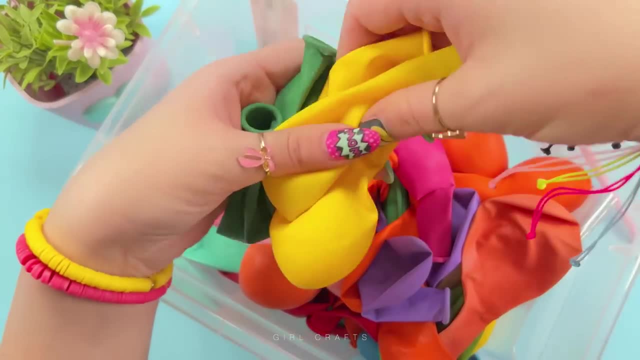 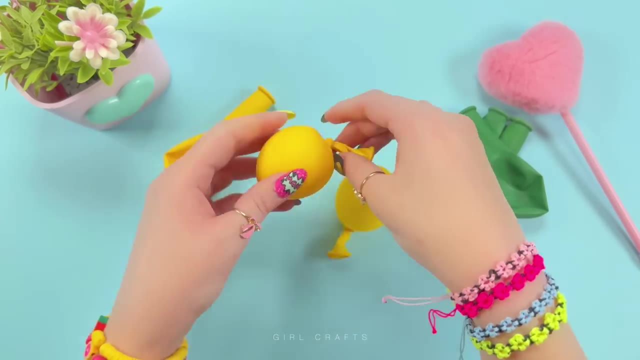 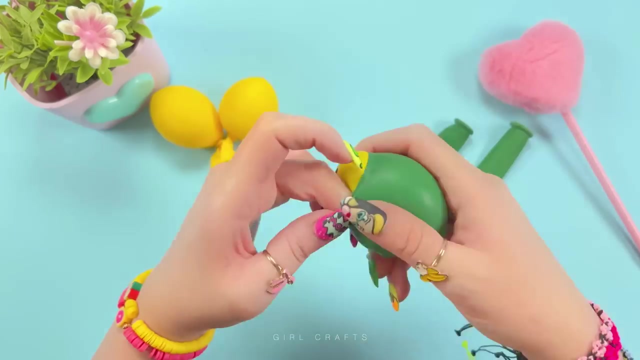 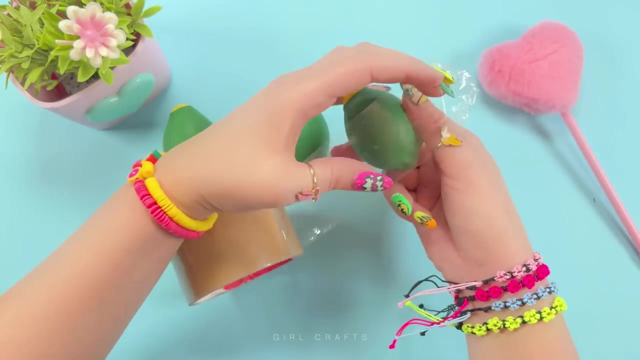 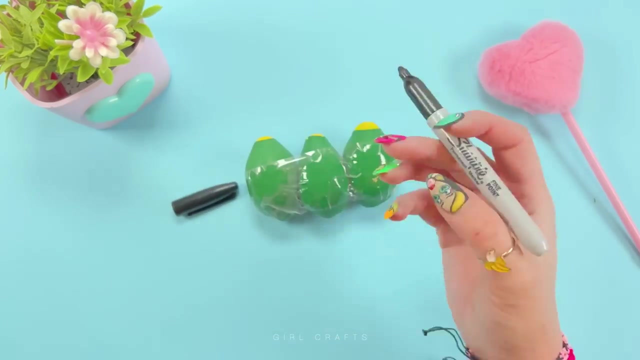 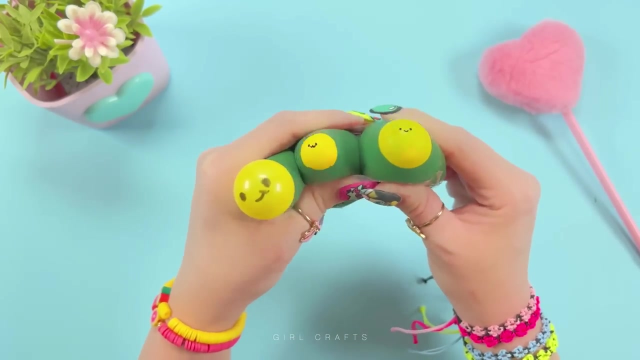 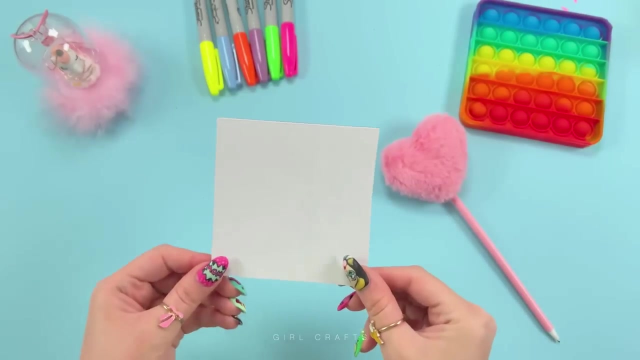 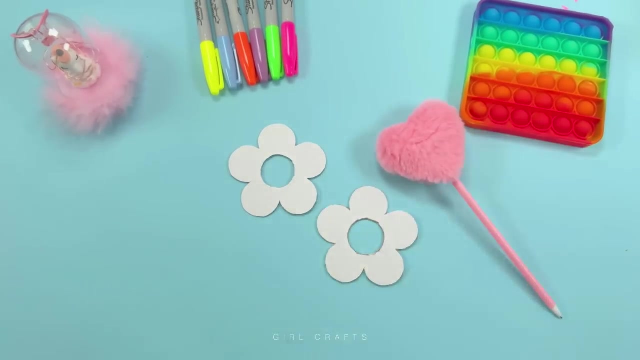 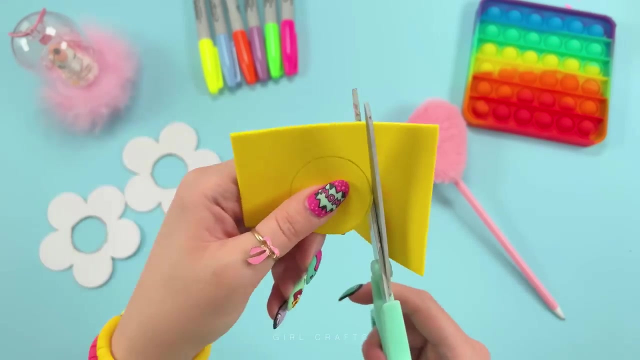 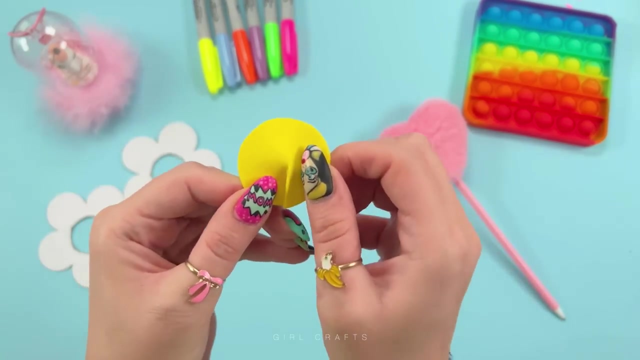 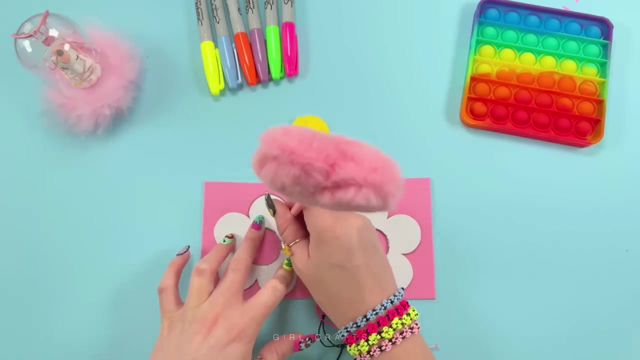 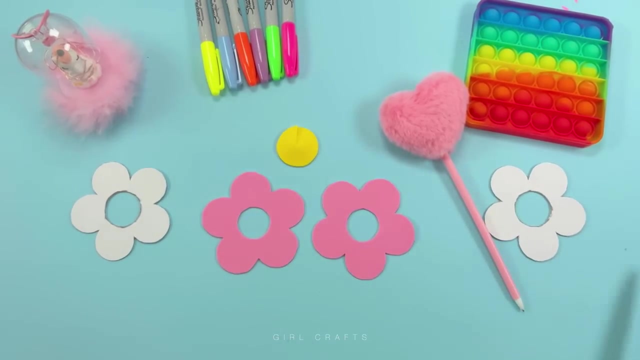 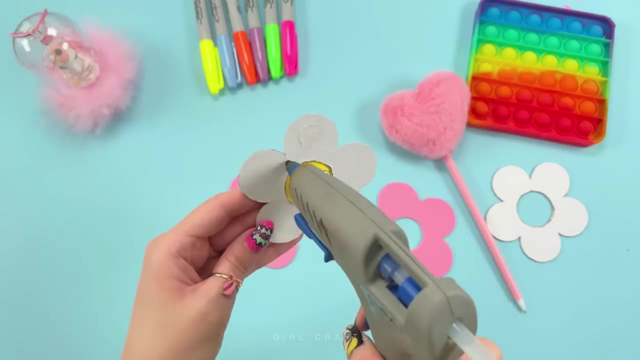 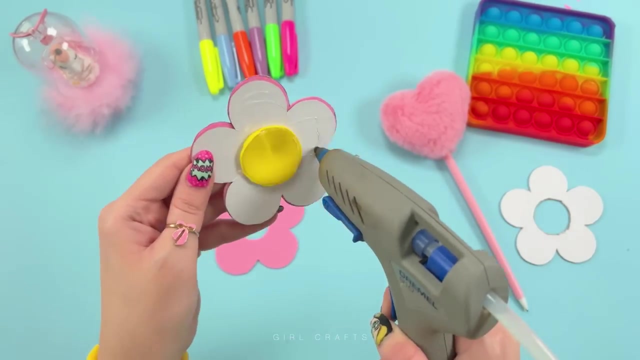 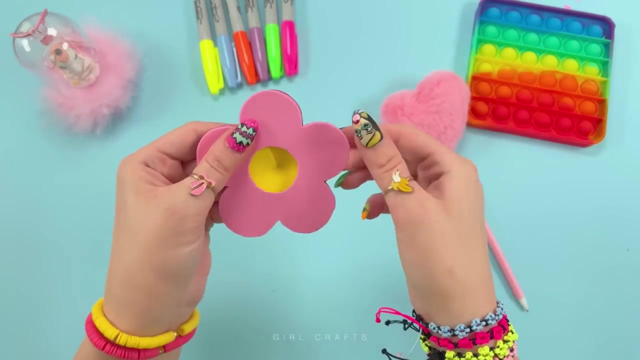 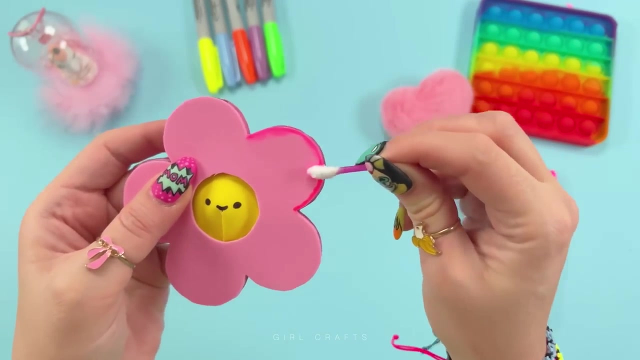 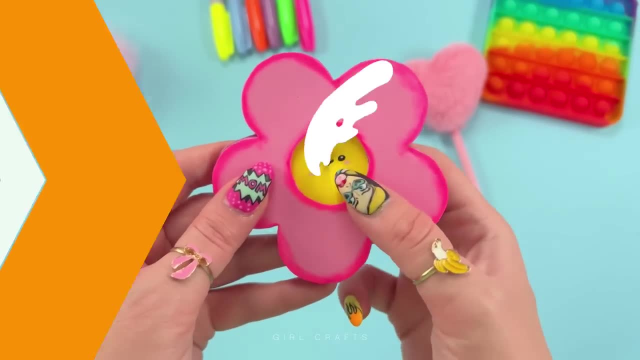 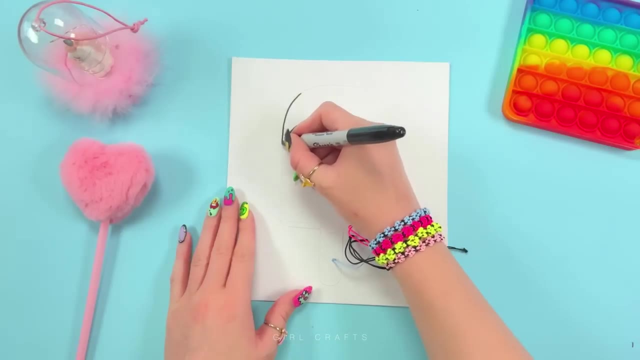 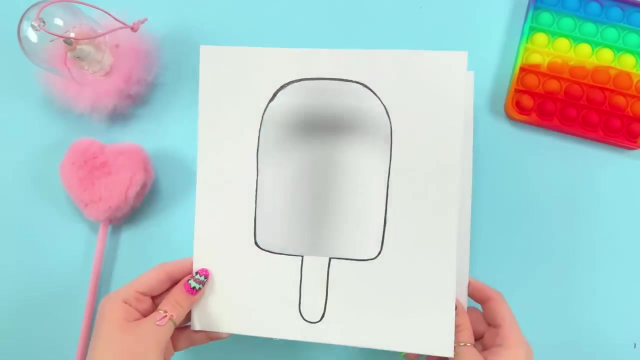 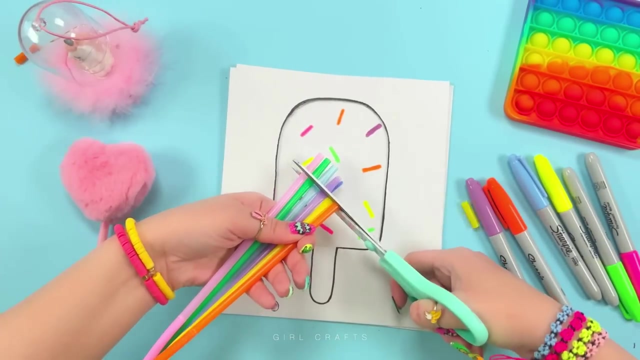 Thank you for watching this video. See you in the next video. Thank you for watching this video. See you in the next video. You say that I'm too worried, Treading just a bit to save, But if I lost you, I would never be the same. 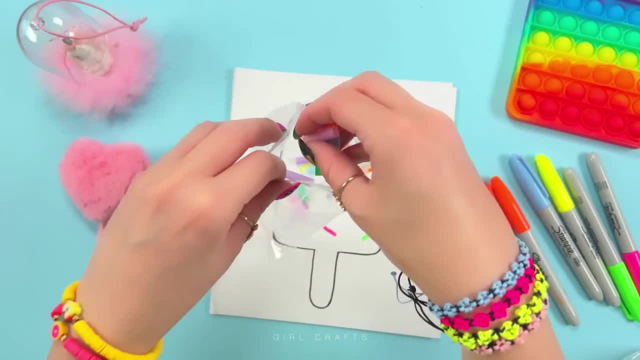 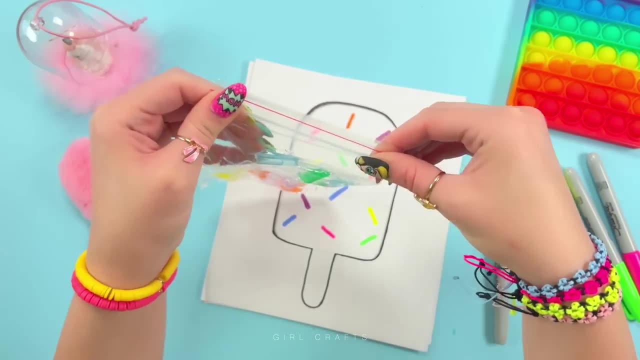 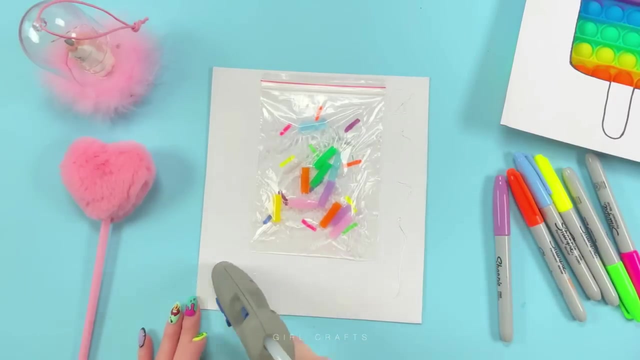 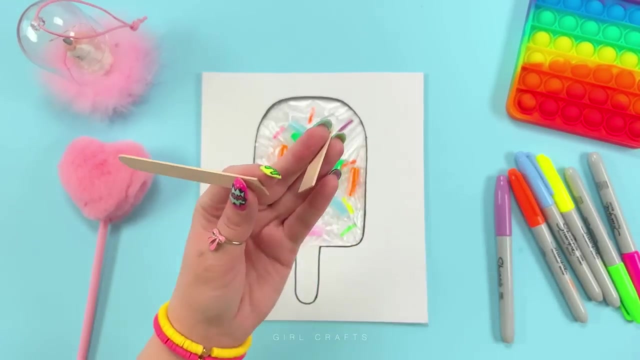 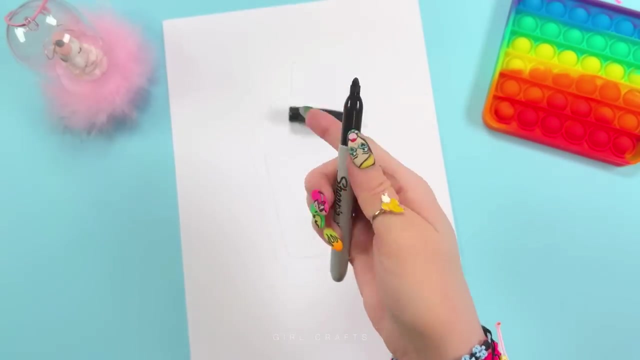 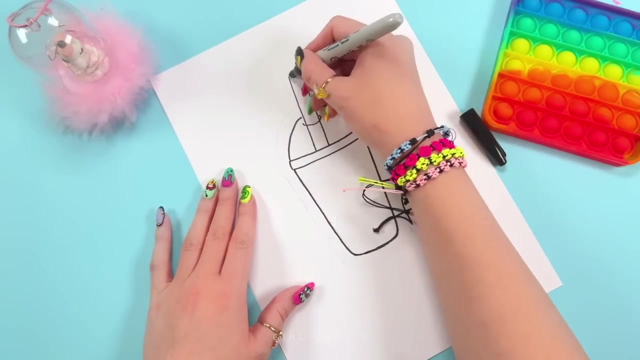 Every song has an ending. Every love is the same. Maybe we'll call us forever, Wishing that this never ends. It's like a dream. It's like a dream when we both get together and feel, Yeah, my mind is spinning, I will never betray. Here is the thing I knew right from the start. 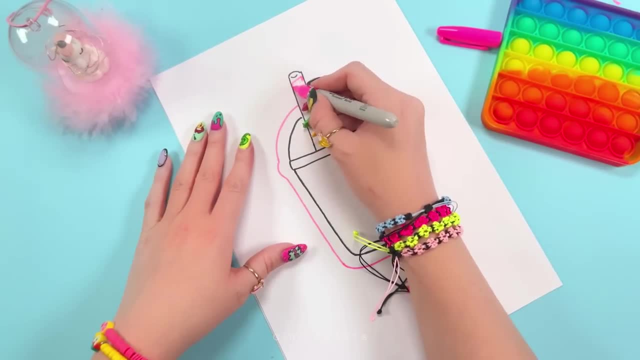 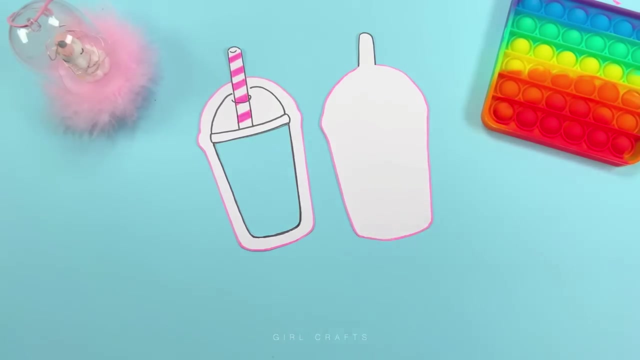 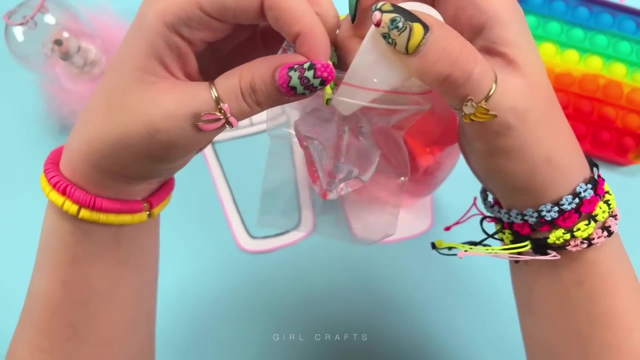 Yeah, you are. you are the best part Of my red heart. You are the best part. Never been this Sure of something in my life. I'll never cool down, Always being in your high. They say that every song has an ending. Every love is the same. 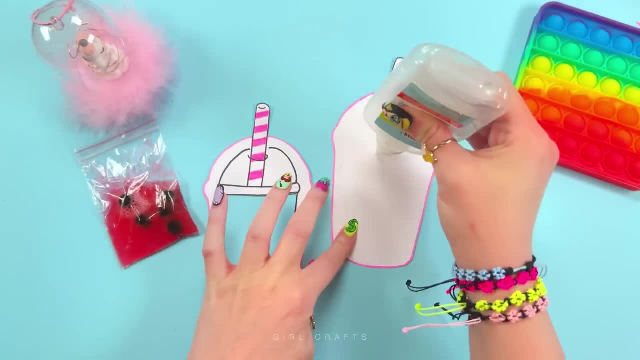 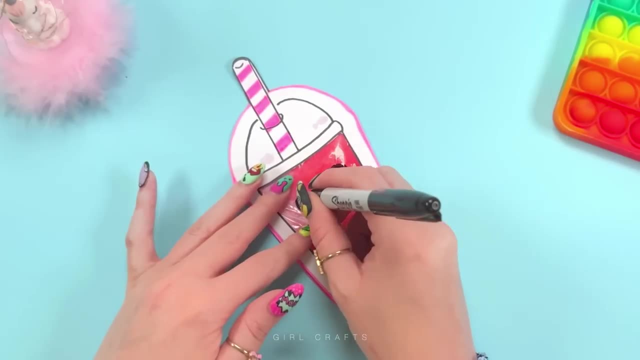 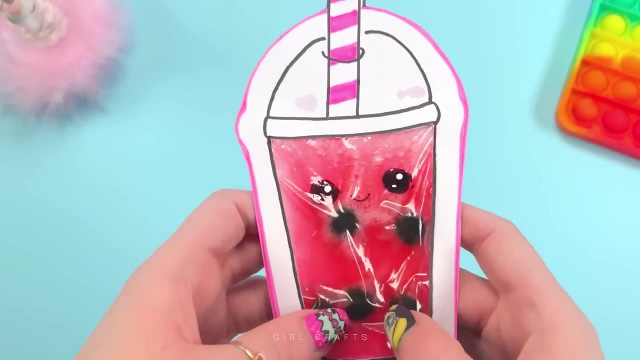 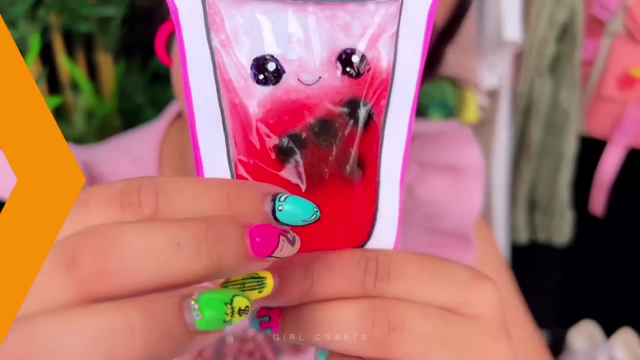 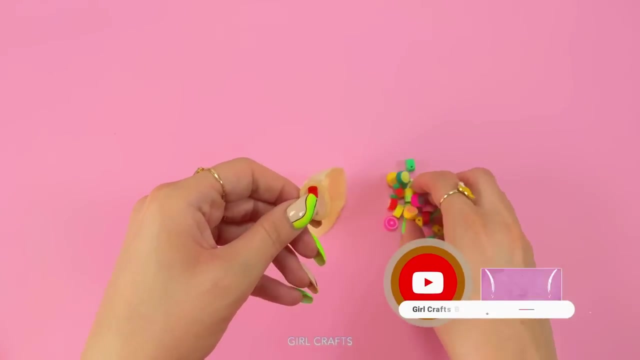 But, baby, we'll call us forever, Wishing that this never ends. It's like a dream. It's like a dream when we both get together and feel, Yeah, my mind is spinning, I will never betray. Here is the thing I knew right from the start. Yeah, you are. you are the best part. 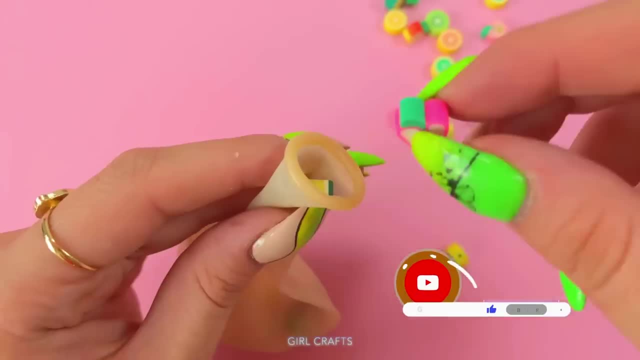 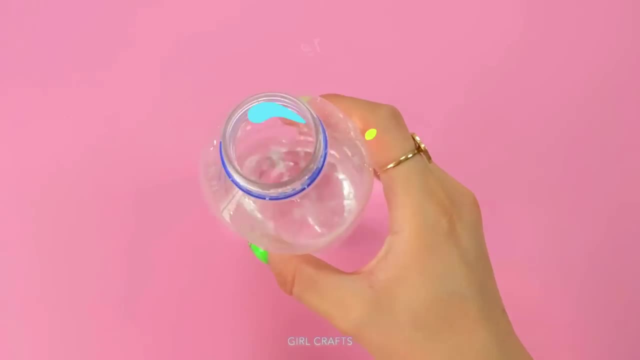 Of my red heart. You are the best part. You are the best part. You are the best part Of my red heart. You are the best part. You are the best part. You are the best part Of my red heart. You are the best part. It's like a dream. 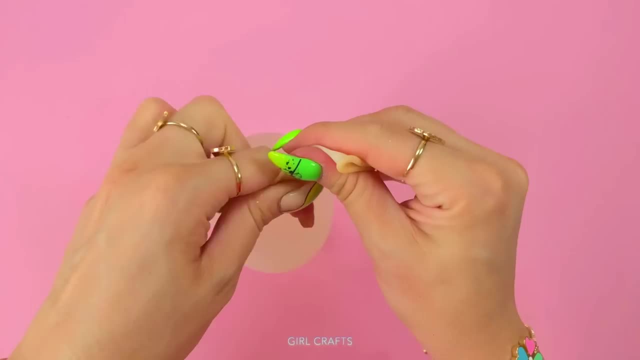 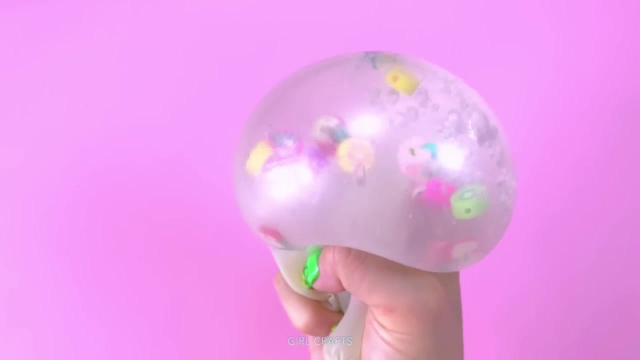 It's like a dream. It's like a dream when we both get together and feel, Yeah, my mind is spinning, I will never betray. Here is the thing I knew right from the start: You are the best part On my red heart, You are the best part. 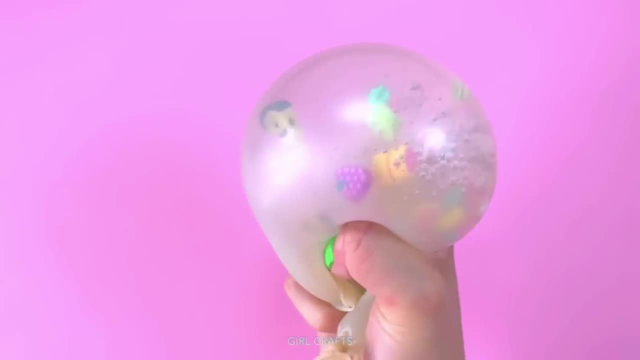 Too damn late To a place where I lost my place In the line to the house of shake, Where I was hoping to find a break. Yeah, Ooh, ooh, ooh, 225 Lucky stars don't achieve the surprise, For this guy has gave me what I like. 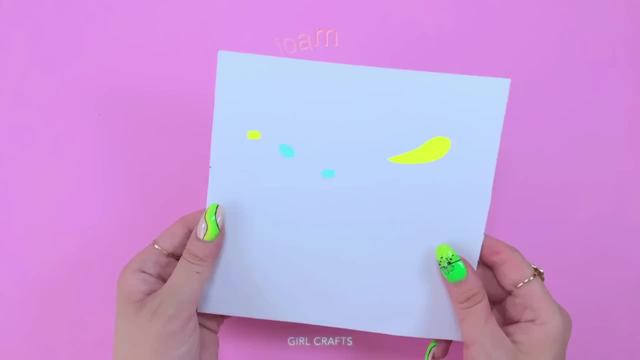 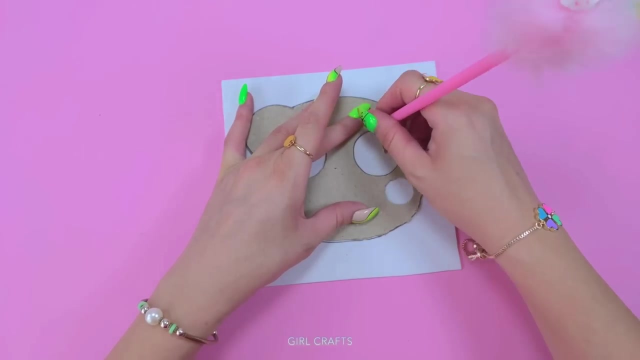 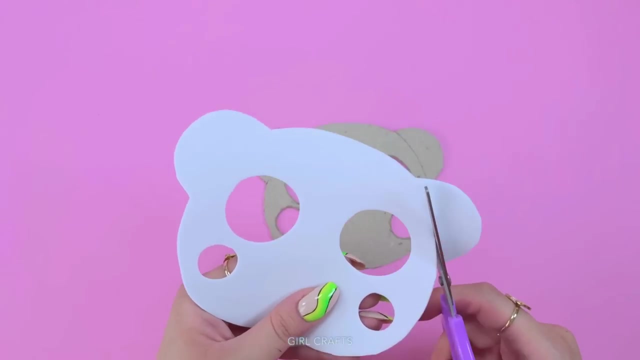 When I slide on our beat while we hide. But I Fell off and it right on my face. yeah, Can't cheer. then start killing bass. yeah, It don't matter, I'm still amazing, I'm fancy. You Don't have to like me, no. 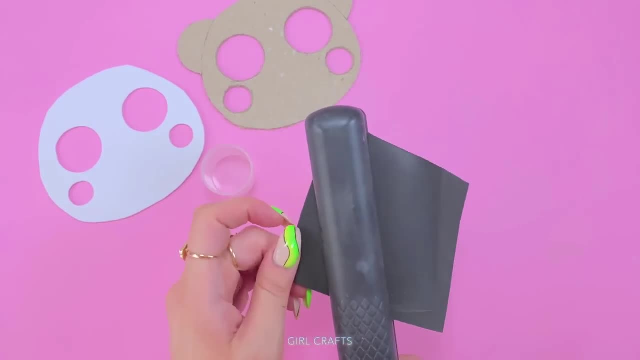 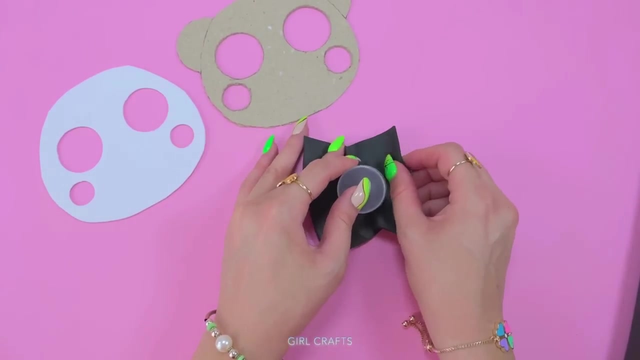 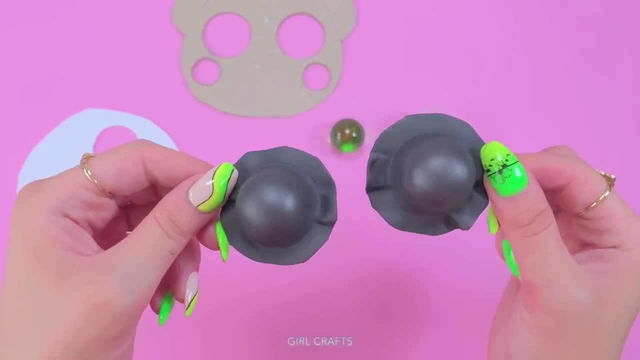 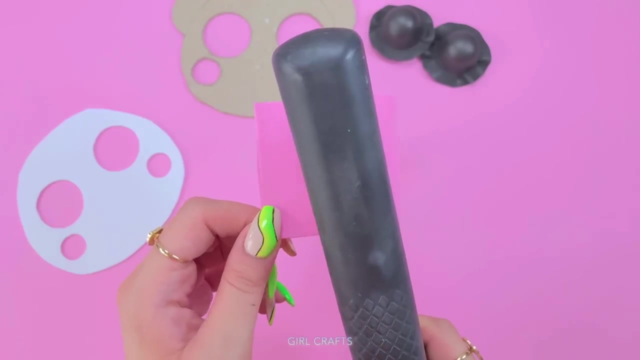 So happy having lost me? yeah, And now we can't be fighting. no, So let it go. Oh, It's off and in Just got home. I've been hovering Round the cool kid company Started to look real promising, yeah. Started to look real promising, yeah. 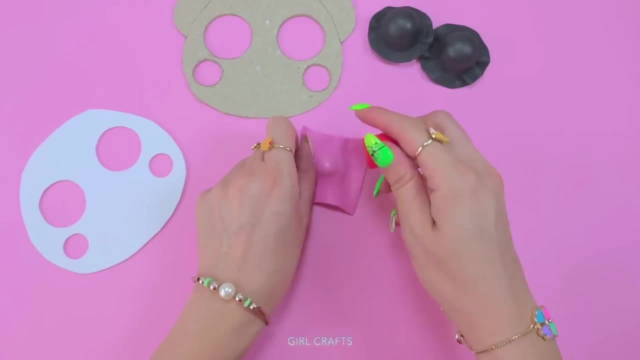 Started to look real promising: yeah, Just so I could live everyday. It's on the tip, don't let it slip. Convincing: yeah, It's on the tip, don't let it slip. The tide keeps sinking in dominion For that place, I found. 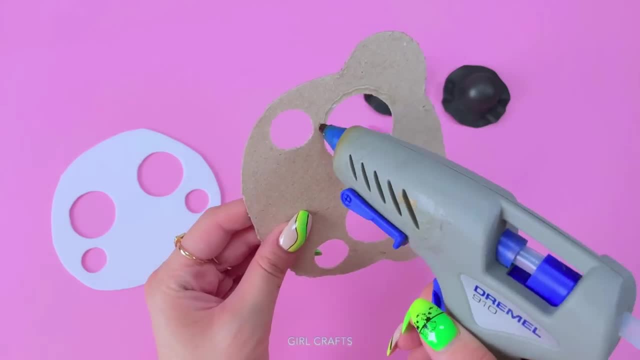 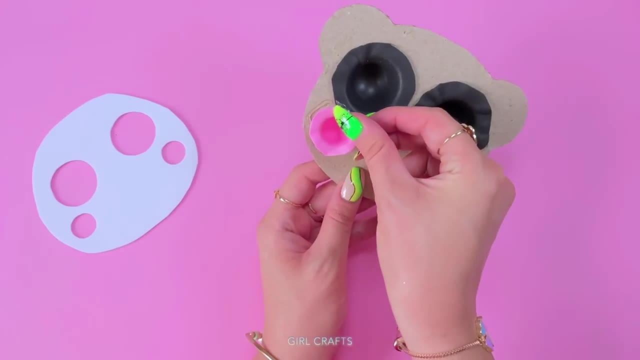 a place to get Ooh, ooh, ooh, 225 Lucky stars. don't achieve the surprise, For this guy has gave me what I like When I slide on our beat every night, But I-I set up and it right on my face, yeah. 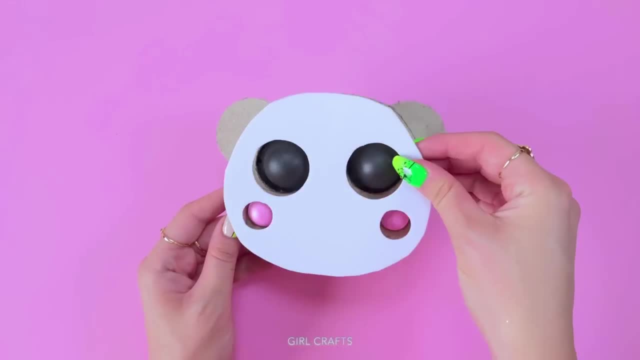 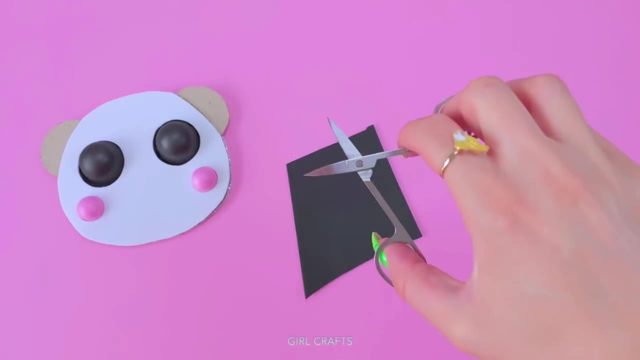 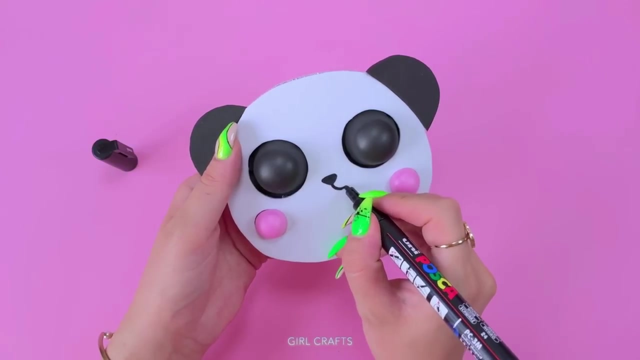 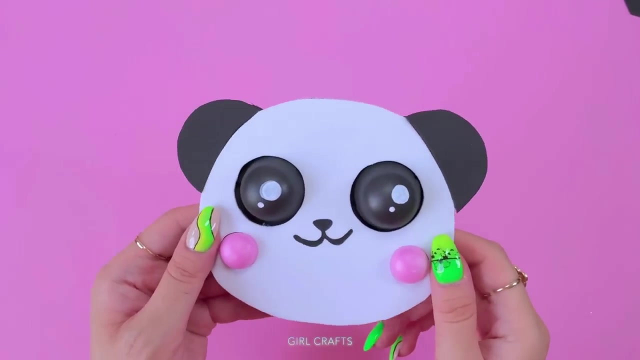 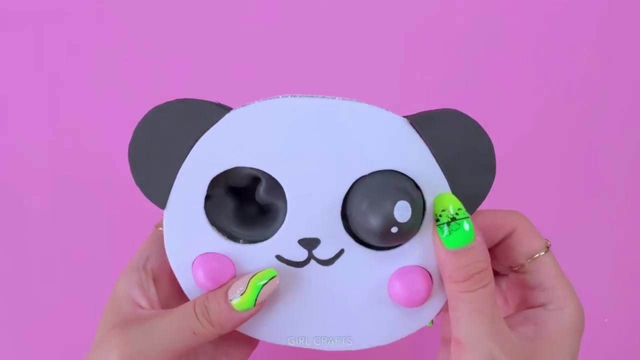 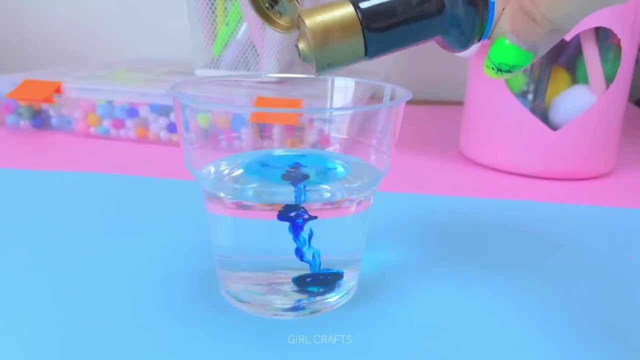 I'm fancy. you don't like me so I'm behind the light. you know I can't be kind to you. so, baby, you know, Fell off, landed right on my face. yeah, Grinchy, then stuck in the base, yeah. 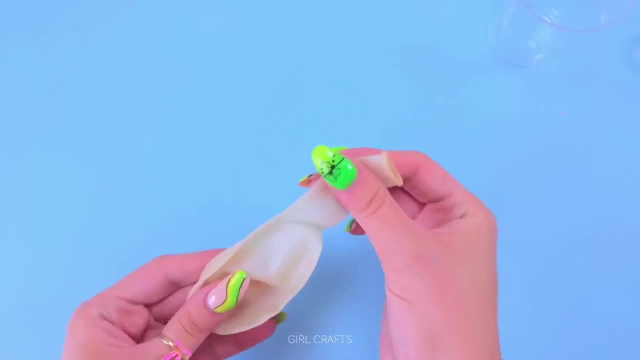 It don't matter, I'm still amazing. I'm fancy. you don't like me, so I can't be kind to you. so, baby, you know I'm fancy. you don't like me, so I'm behind the light. you know I can't be kind to you. so, baby, you know. 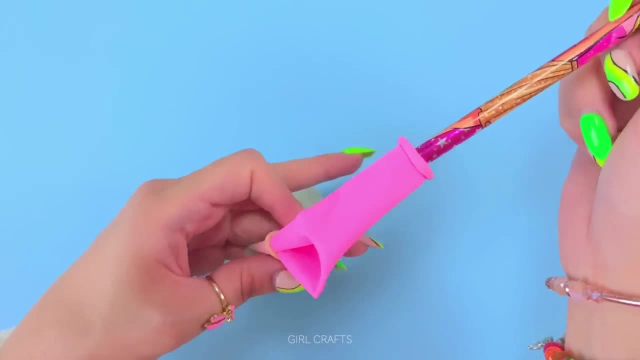 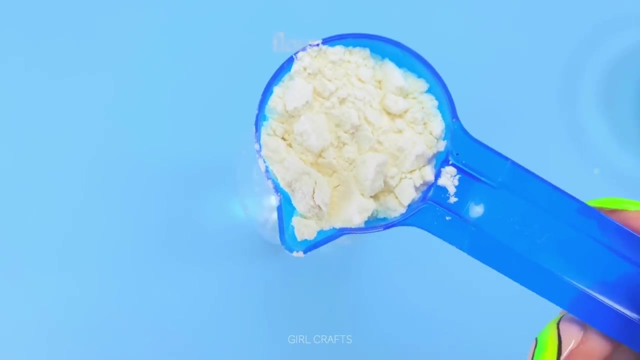 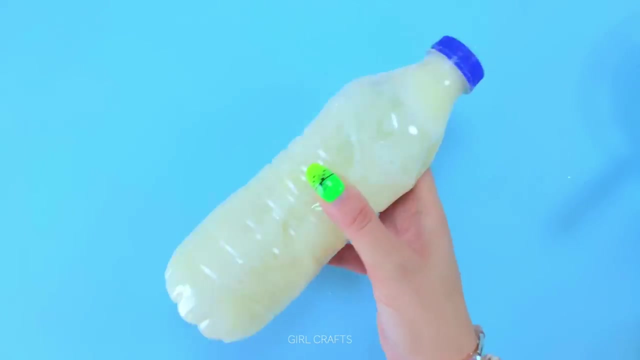 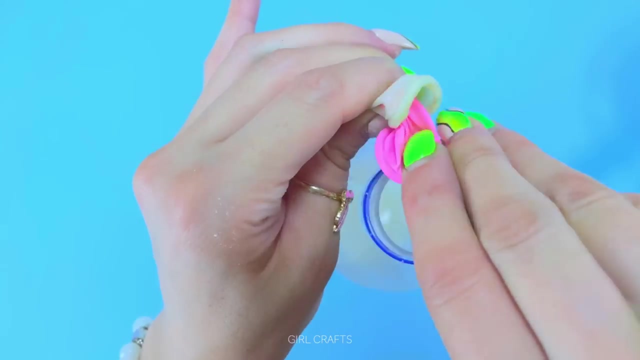 It don't matter, I'm still amazing, I'm fancy. you don't like me, so, baby, you know I don't wanna be the girl, but I kinda need a word. well, I'm into you And all I know. it's been a long time. I was on the sideline waiting for you. 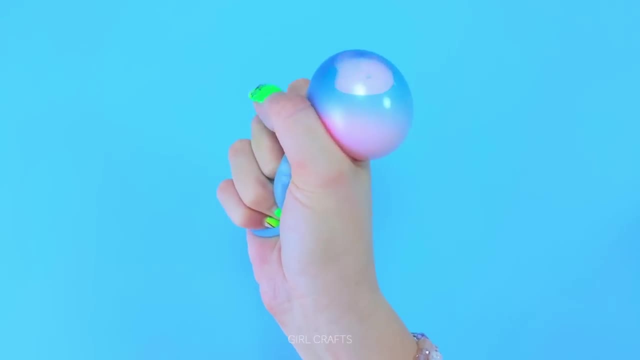 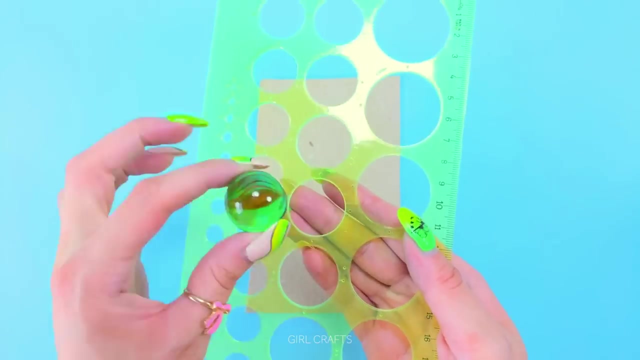 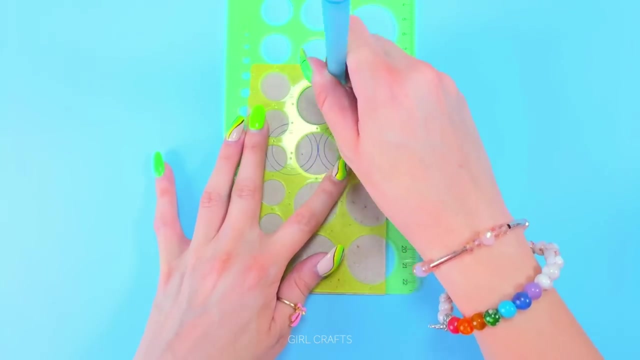 We could go to California or anywhere you wanna. as long as I'm with you, I'm alright. And we don't need the drama. we'll find our own nirvana. so run away with me. We don't need the drama, we'll find our own nirvana. cause it feels like I'm dreaming. 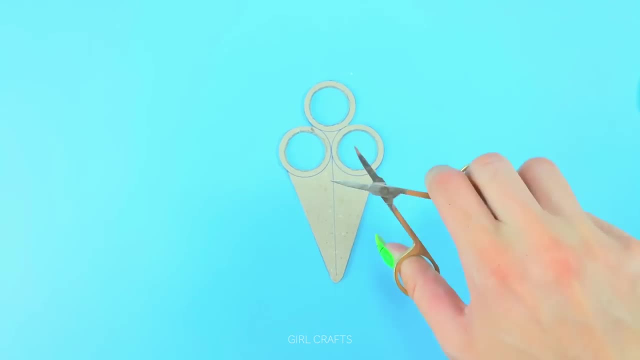 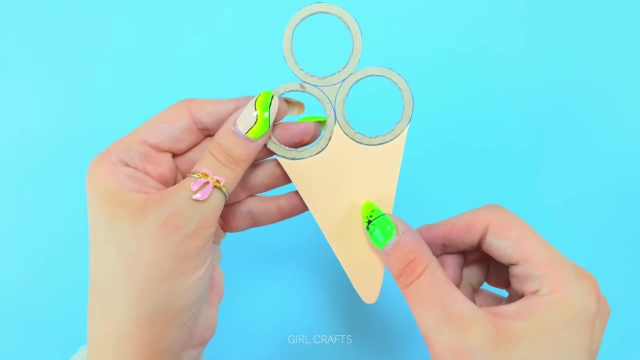 When I'm waking up next to you And my whole heart is beating because it's beating next to you. Let's find something better to hold on to cause we can do anything we want to, And I can't help the feeling that I get when I'm with you. 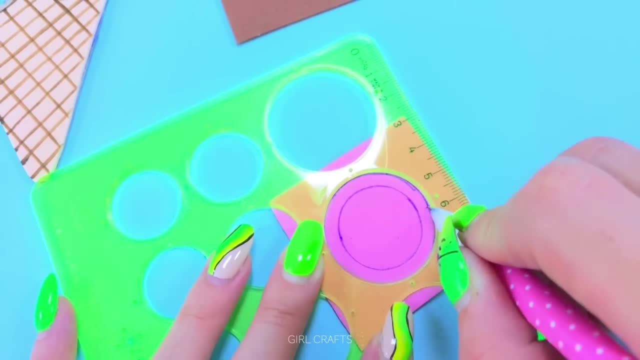 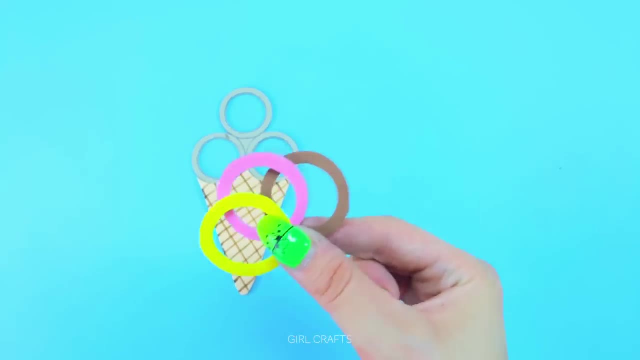 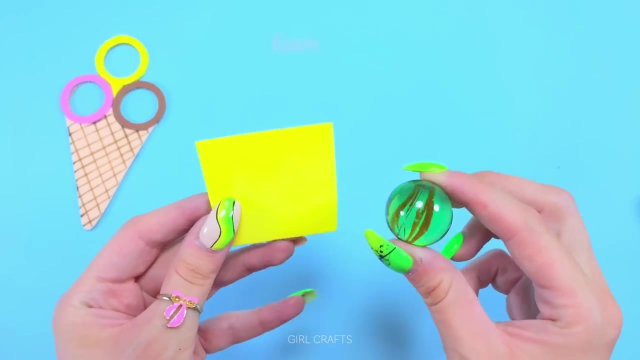 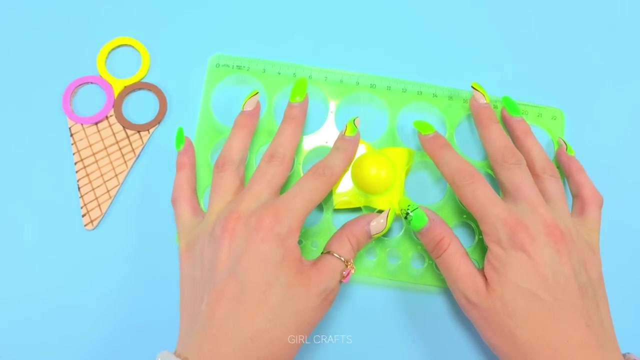 When I'm waking up next to you. You just gotta make your mind up. just give me a sign if you want a ride. They don't really wanna know, so we throw away our phones, go bunny and glide. We could go to California or anywhere you wanna. as long as I'm with you, I'm alright. 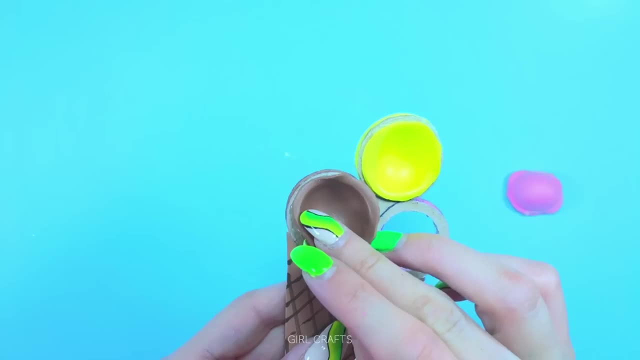 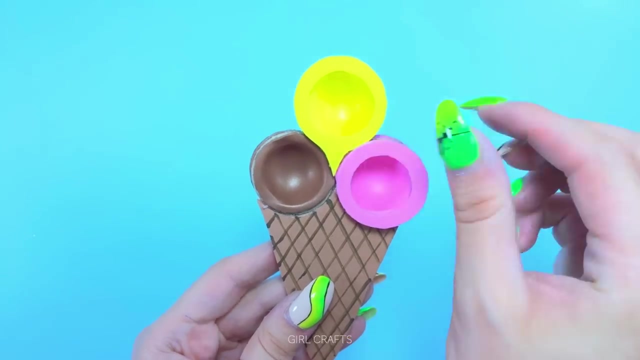 You could go to California or anywhere you wanna. as long as I'm with you, I'm alright. And we don't need the drama. we'll find our own nirvana. so run away with me tonight, Cause it feels like I'm dreaming when I'm waking up next to you. 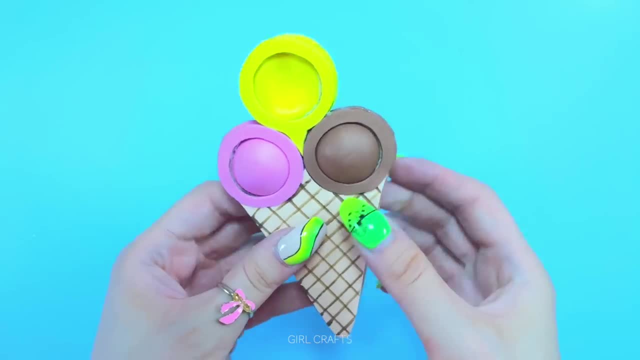 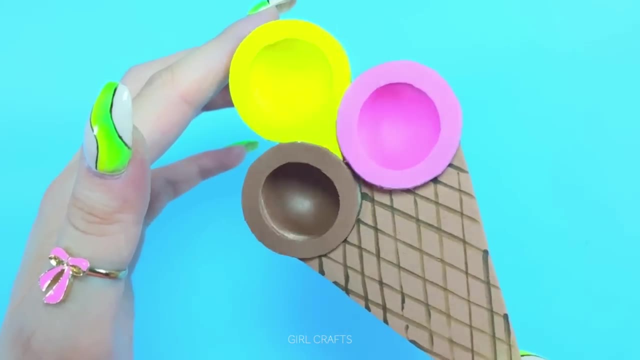 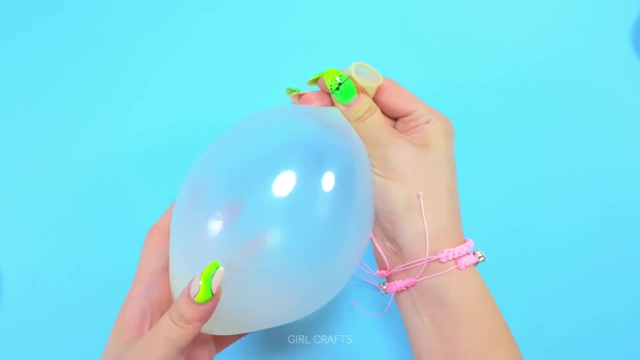 And my whole heart is beating cause. it's beating next to you. Let's find something better to hold on to, cause we can do anything we want to. We want to, And I can't help the feeling That I get when I'm next to you. Tonight we're running on the right track. I know we never gonna look back. Oh, I just wanna have a good time. Call me whatever, Cause I'm up for anything like that. Oh no, we don't wanna do no more, So tonight we'll just let go. 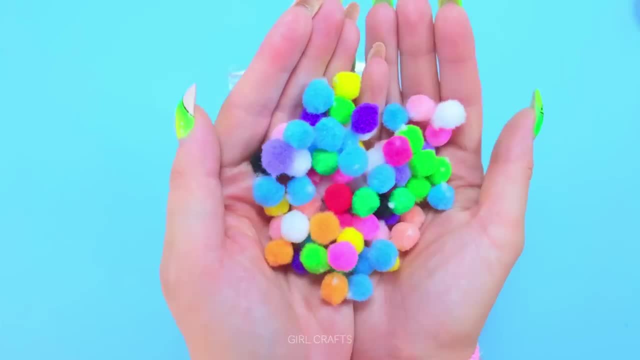 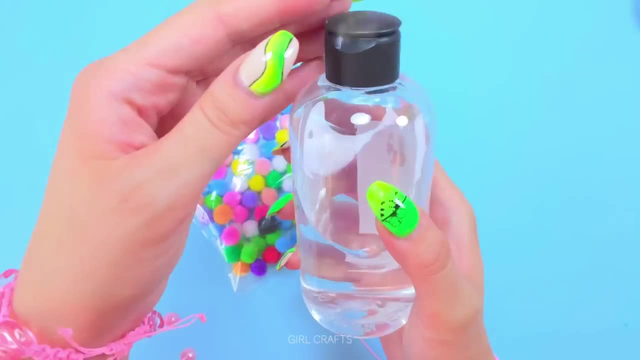 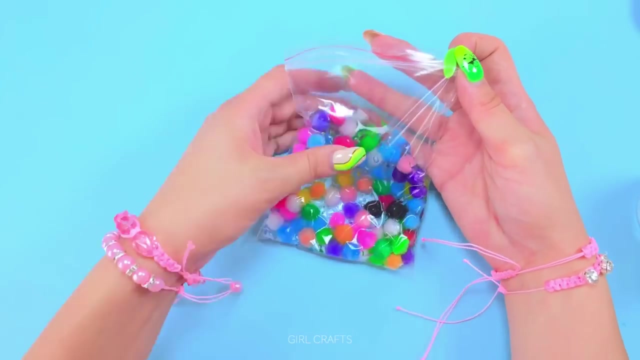 To the beat and the street And we'll freak out singing like Singing, like Party, like Freaking out To the beat, and we'll freak out Singing like Singing, like Party, like Freaking out To the beat, and we'll freak out To the beat and we'll freak out. 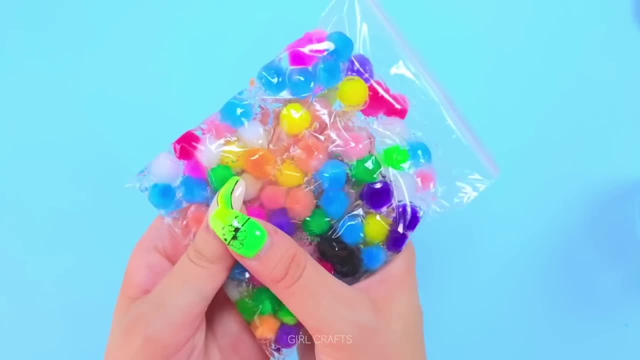 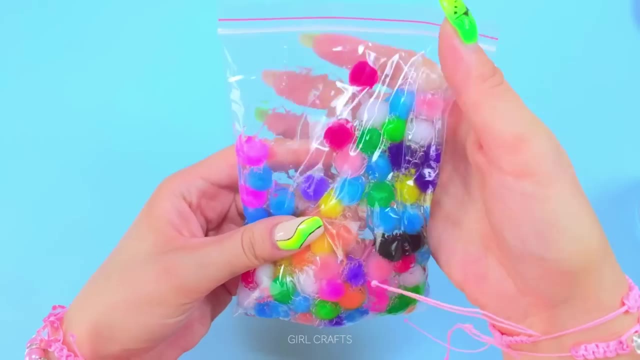 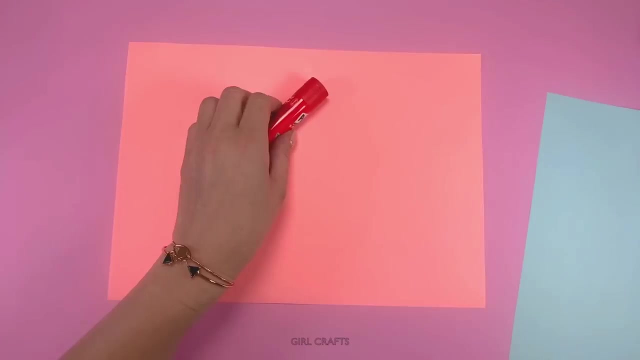 To the beat and we'll freak out Singing like Wasting fun in doing what you're told. I don't mind, even though I lose control. Oh, I just wanna have a good time, So call me whenever, Cause a night like this, it never gets old. Oh no, we don't wanna do no more. So tonight we'll just let go To the beat and the street And we'll freak out singing like Freaking out Party, like Freaking out To the beat, and we'll freak out Singing like Freaking out. 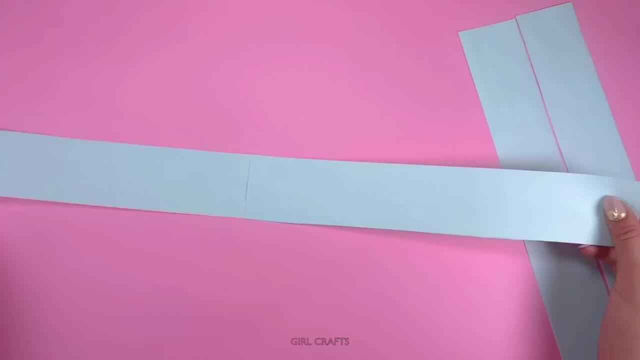 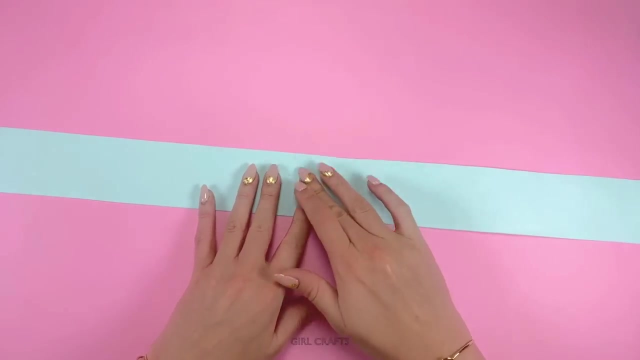 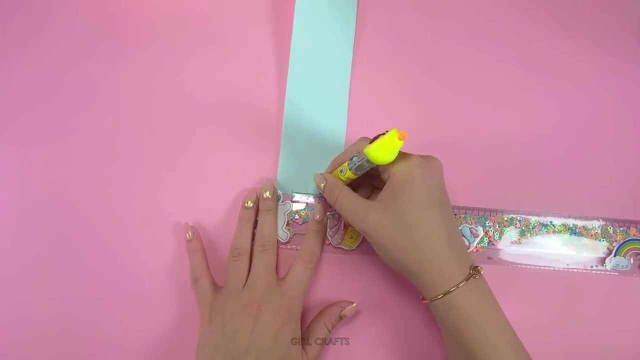 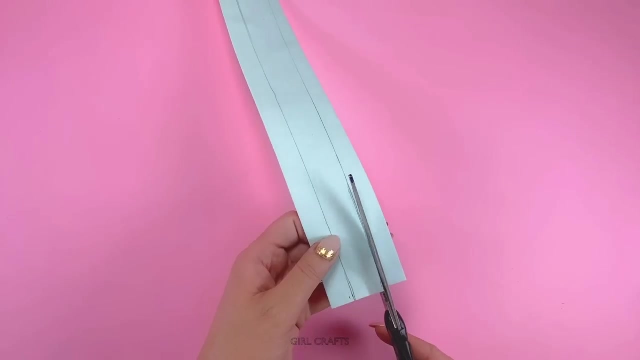 Party, like Freaking out To the beat and we'll freak out Singing, like: So, baby, come and take my hand tonight And know that everything will be alright When we dance and we fall, And we don't care at all. Now we just sing the La-la-la-la-la-la-la-la-la-la-la. 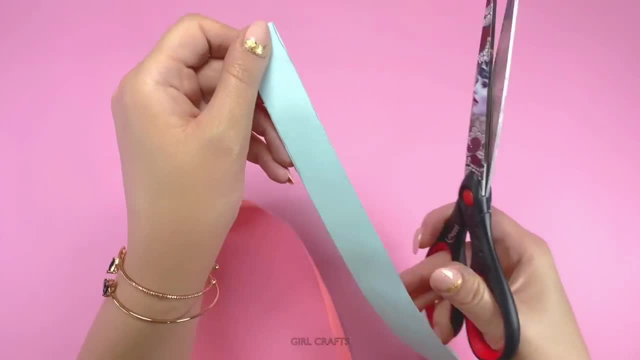 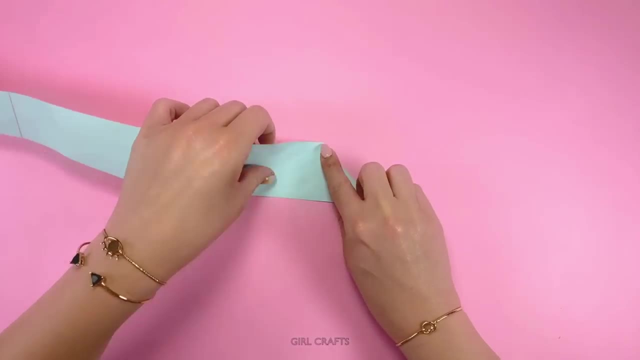 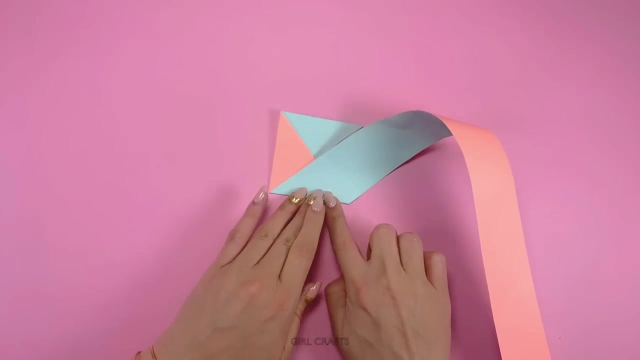 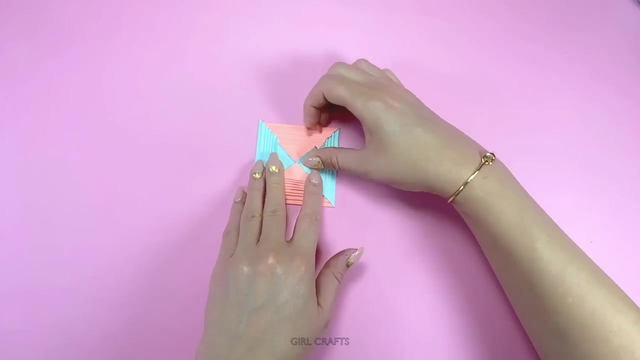 La-la-la-la-la-la-la-la-la-la-la-la-la-la-la-la-la-la-la-la-la-la-la-la-la-la-la-la-la-la-la-la-la-la-la-la-la-la-la-la-la-la-la-la-la-la-la-la-la-la-la-la-la-la-la-la-la-la-la-la-la-la-la-la-la-la-la-la-la-la-la-la-la-la-la-la-la-la-la-la-la-la-la-la-la-la-la-la-la-la-la-la-la-la-la-la-la-la-la-la-la-la-la-la-la-la-la-la-la-la-la. 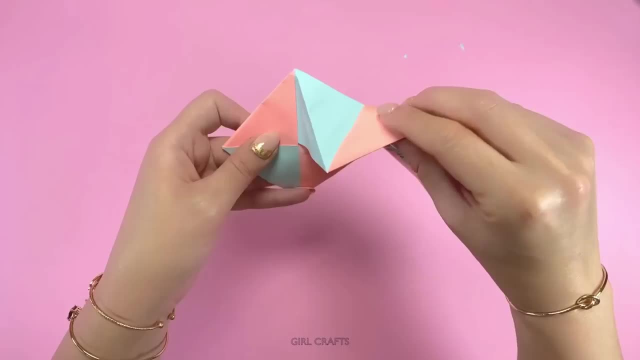 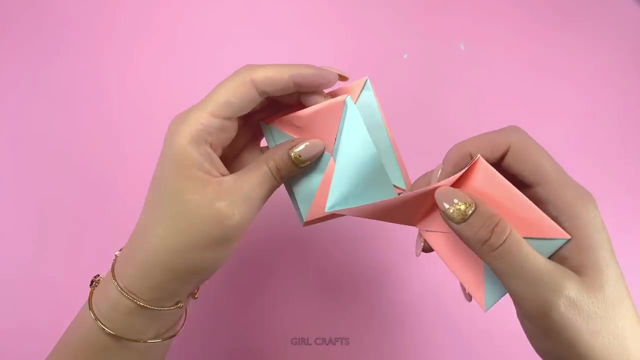 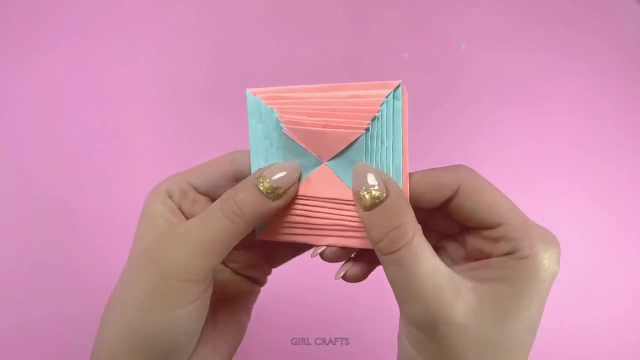 La-la-la-la-la-la-la-la-la-la-la-la-la-la-la-la-la-la-la-la-la-la-la-la-la-la-la-la-la-la-la-la-la-la-la-la. Lights down low, still wondering what you're saying. Stay, stay, stay. 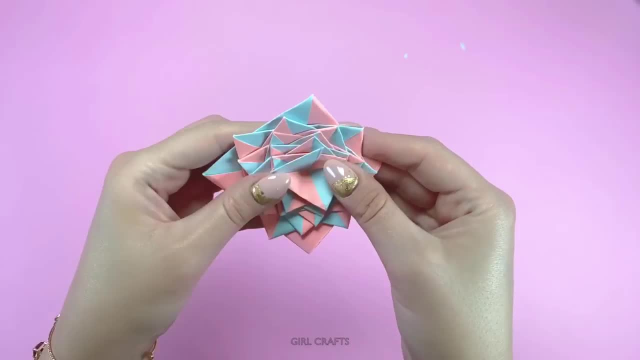 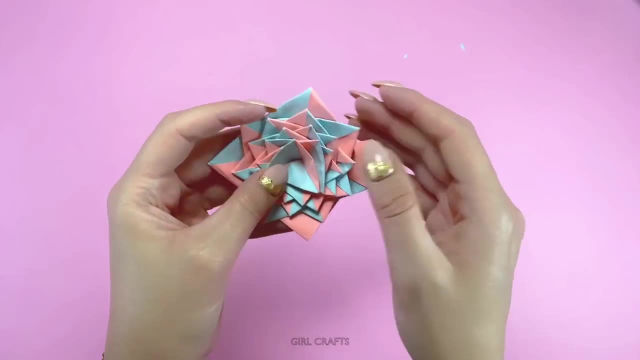 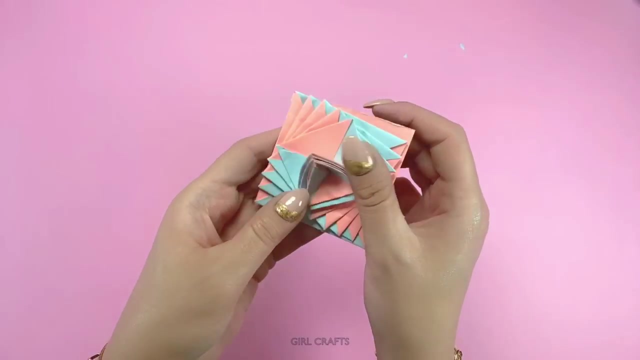 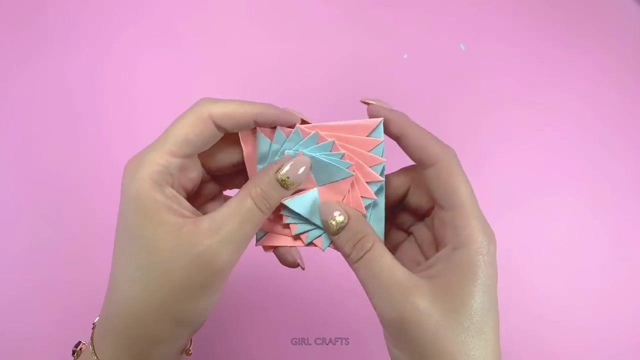 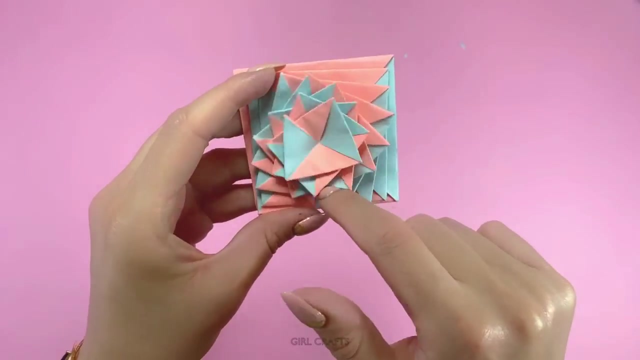 Baby, please don't go. I'd rather have you stayin'. Stay, stay, stay, stay. Pick up the mess that you left shattered on the floor. Keep the lights down low. What is this game you're playing? Don't get me wrong, I'm all ready. for what? 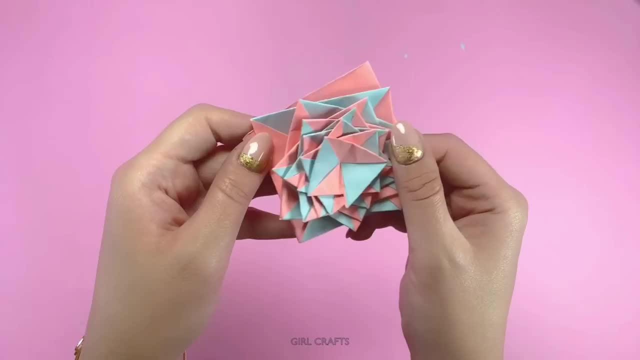 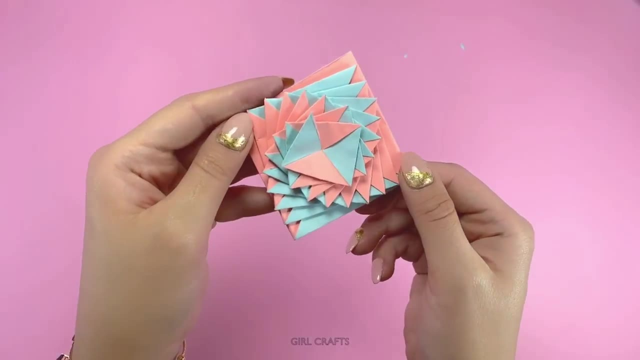 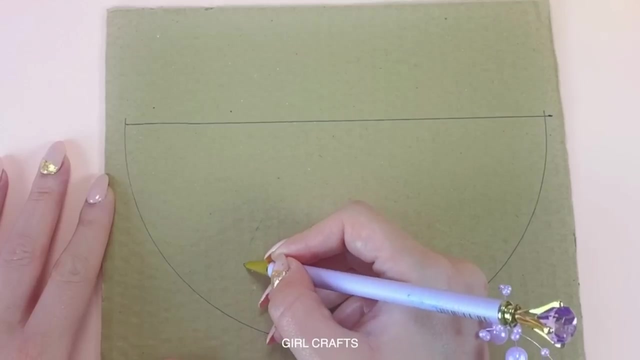 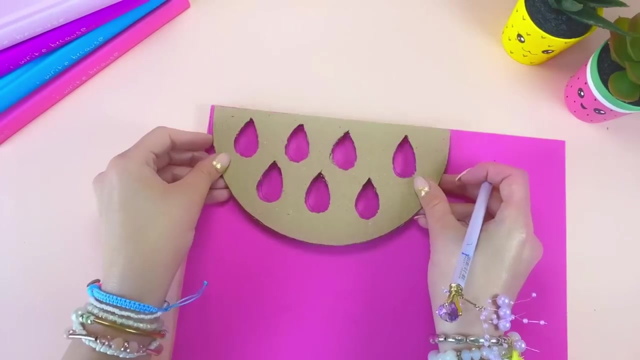 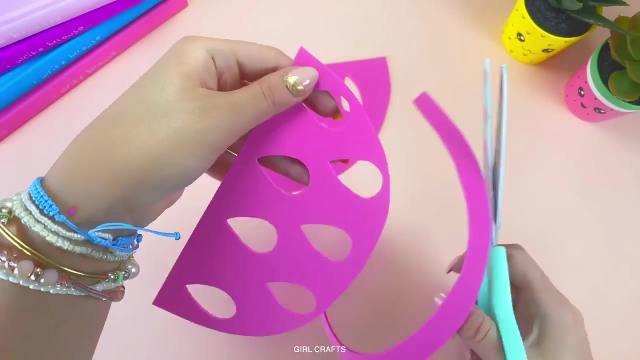 Future is lying ahead of us, Cause I want you need your hair right on my shoulder. Please stay, just stay for now. It's 3.2 from the driveway of my house To your apartment where I am waiting. Now, come on, don't think night's young. 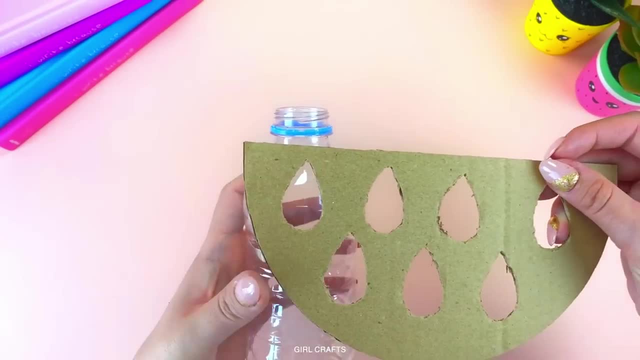 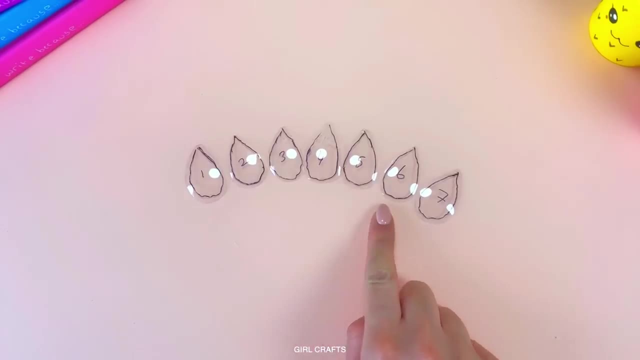 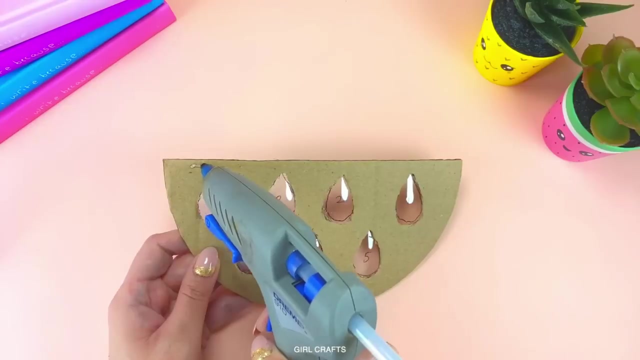 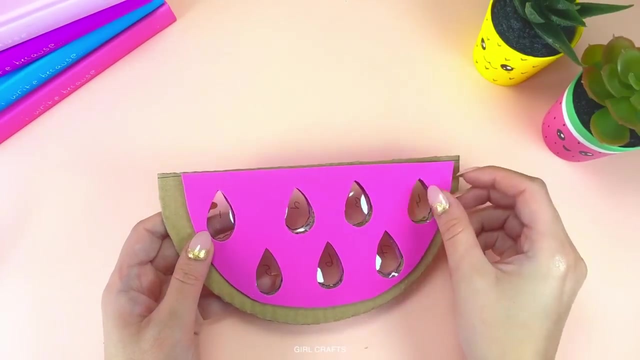 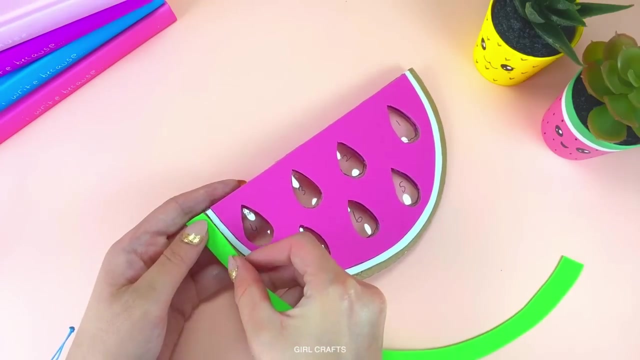 Let's go. NYC, Portland, Austin, Anaheim, Maybe not Anaheim. Keep an open mind. I'm just saying: baby, Let's go, I don't care Anywhere. Like a river connects to the ocean, This baby touches wherever We're going. White lines flying by, Who knows what we'll find. 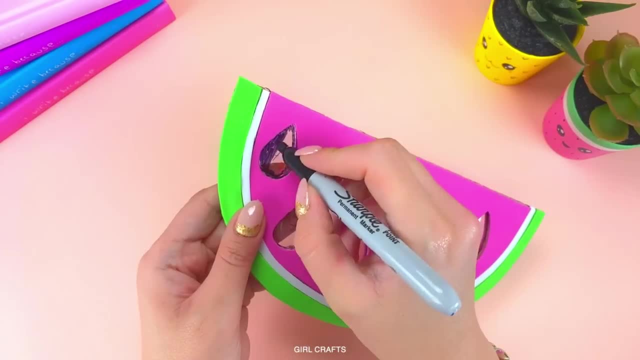 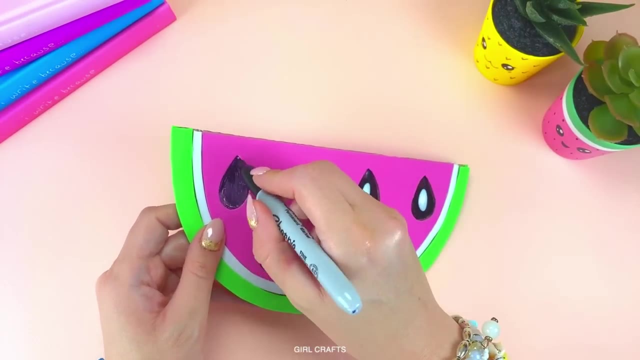 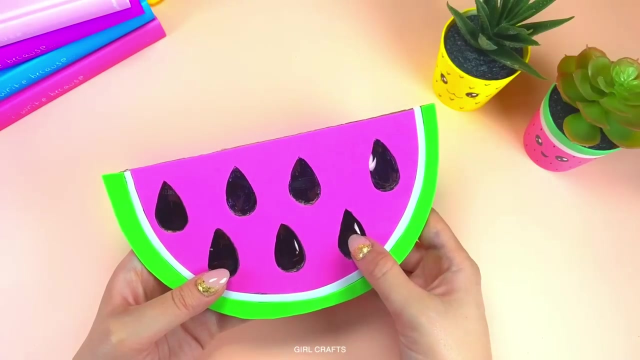 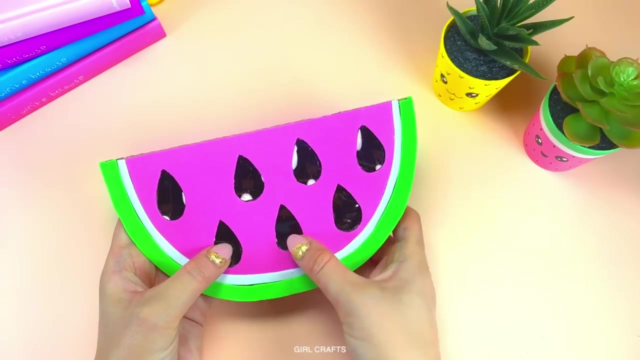 You and me tonight, Try, Let's try. When's the last time we dropped our things and went Woke up somewhere that we've both never been? Growing up doesn't mean getting older. Maybe it's just left. time Turns off familiar streets. I just wanna come back with a memory. 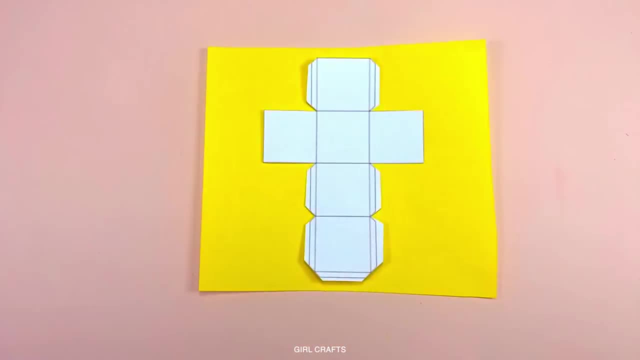 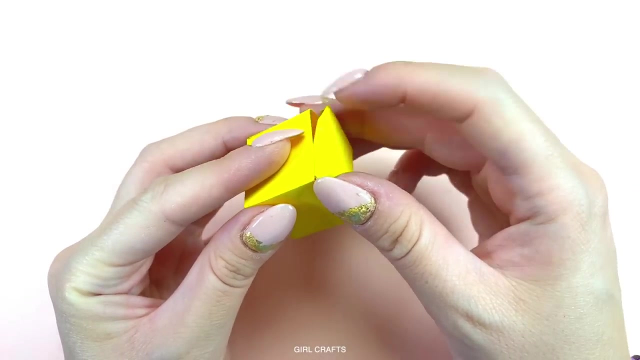 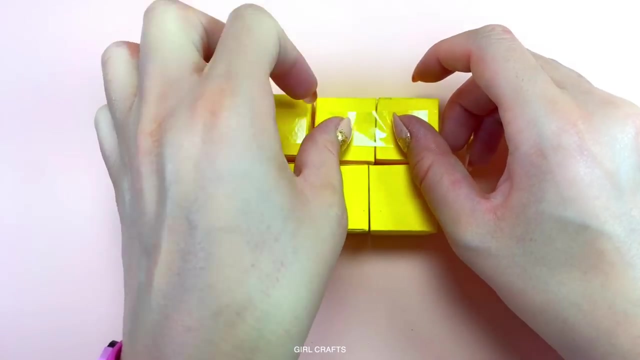 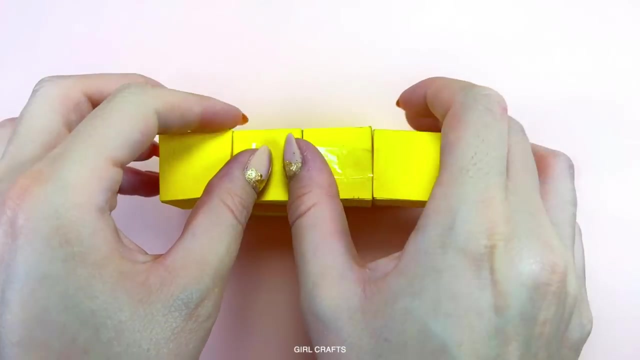 Growing up doesn't mean getting older. I don't care Anywhere. Like a river connects to the ocean, This baby touches wherever we're going, White lines flying by Who knows what we'll find. You and me. tonight We'll be together at this place, Our first meeting. Tonight, Let's drive, Let's drive, Let's drive. Remember When we were young and free. Oh, the way it used to be. Tell me, can we go back? Oh, the way it used to be. Tell me, can we go back? Oh, the way it used to be. 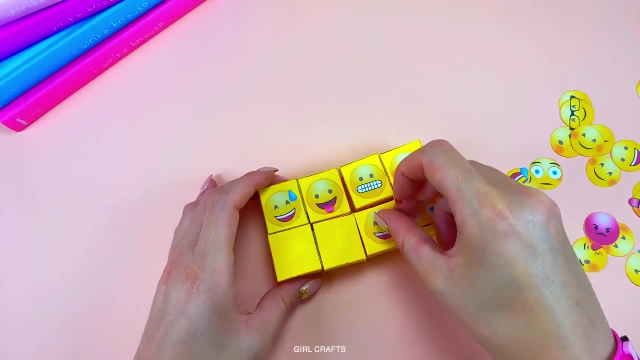 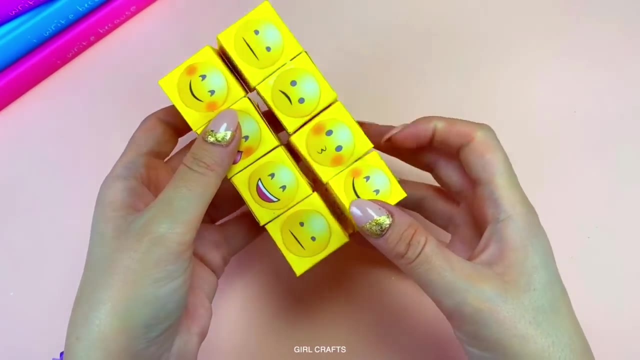 Tell me, can we go back? Sweet night, at the end of the tunnel, We were alone in the car. We were alone in the car From the driveway of my house To your apartment where I am waiting now. Like a river connects to the ocean This pain. it touches wherever we're going. 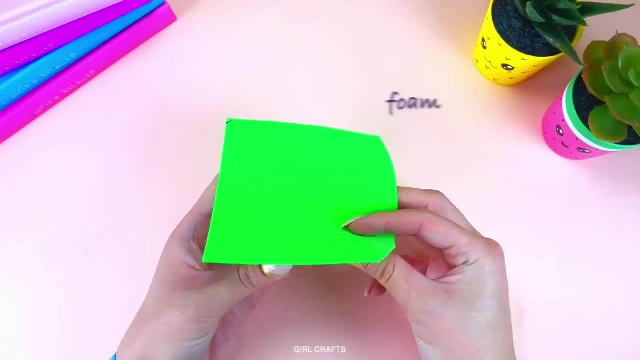 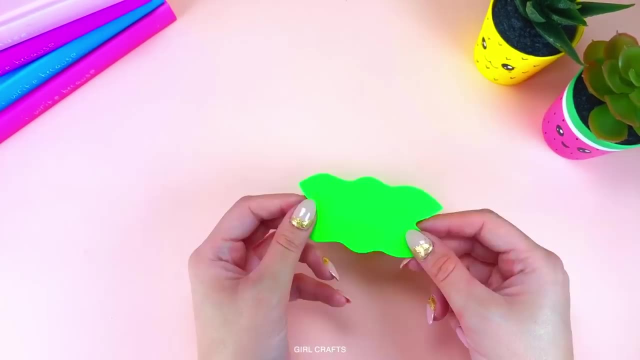 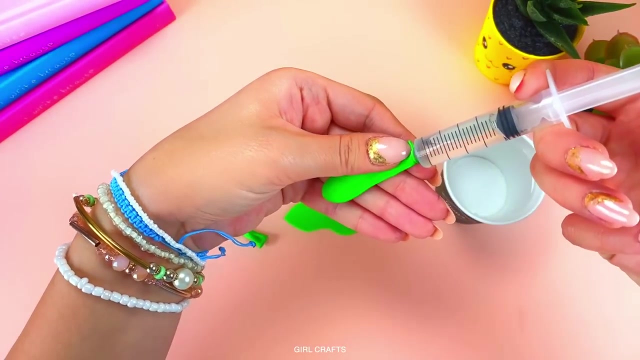 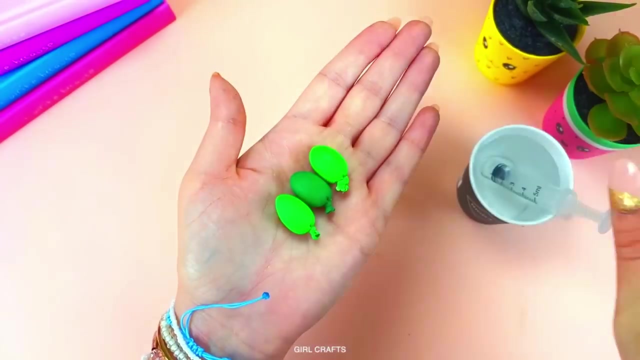 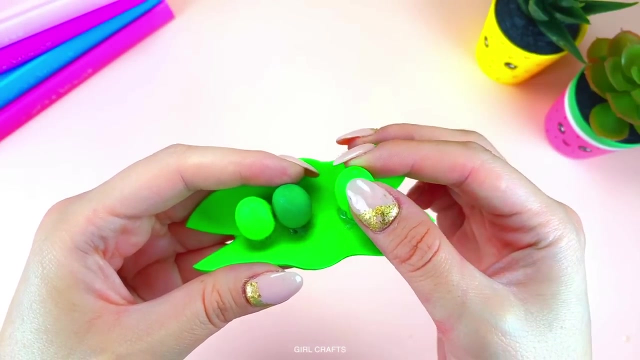 White lines flying by. Who knows what we'll find You and me tonight. Like a river connects to the ocean. This pain, it touches wherever we're going. White lines flying by. Who knows what we'll find You and me tonight. Yeah, let's try. Let's try. 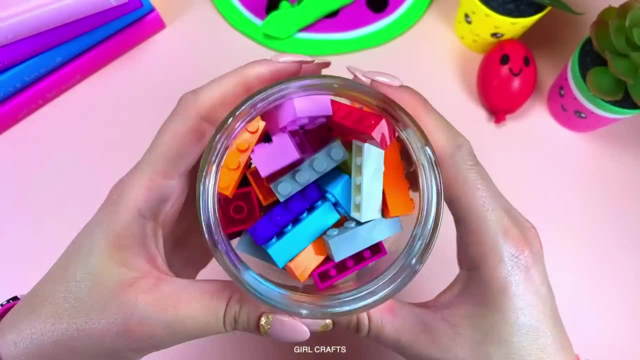 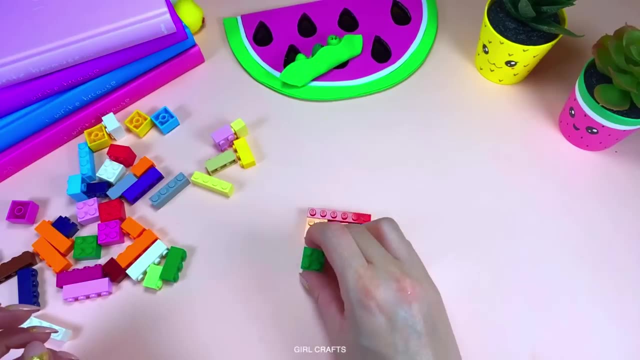 Looking in the mirror. who's she? Oh wait, that's me. that's me. Who's the pretty thing that I see? Yeah, that's right, that's me, that's me. I'm not trying to sound bougie, But I'm rocking it. VIP. 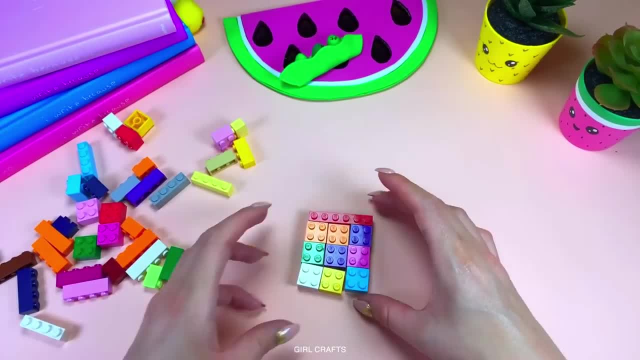 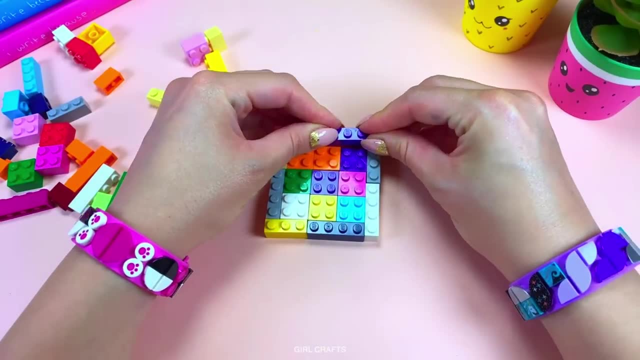 I'm the one they're trying to beat. Wanna get on my team? That's right. that's me. that's me. Got my swag on max Throwing hot sauce on the tracks. Got my swag on max Throwing hot sauce on the tracks. 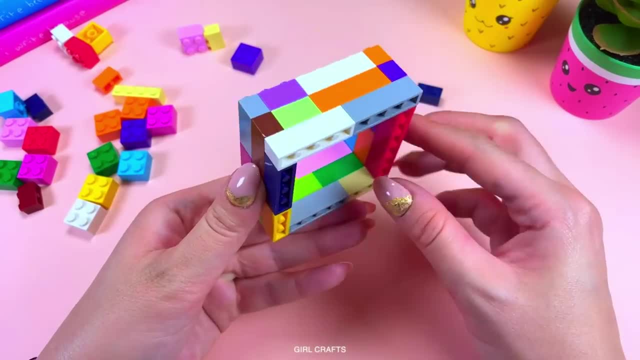 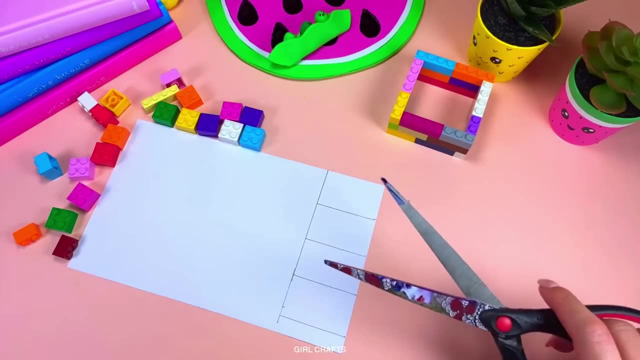 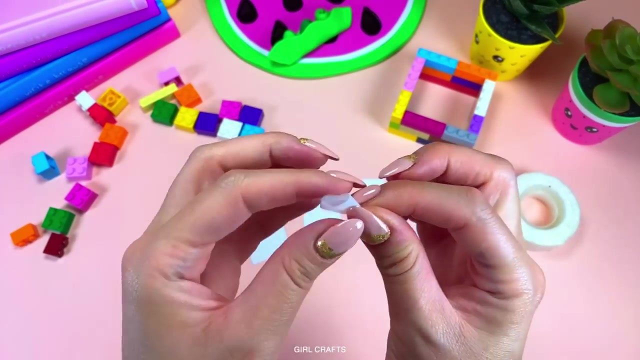 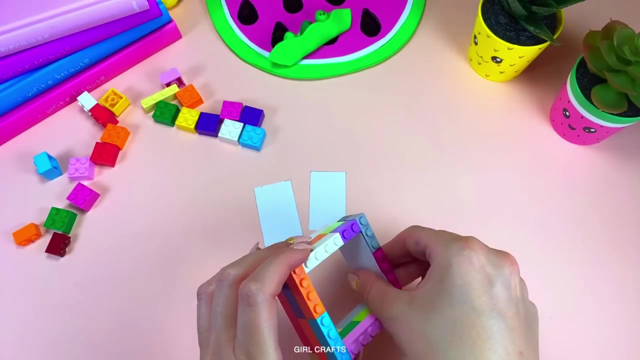 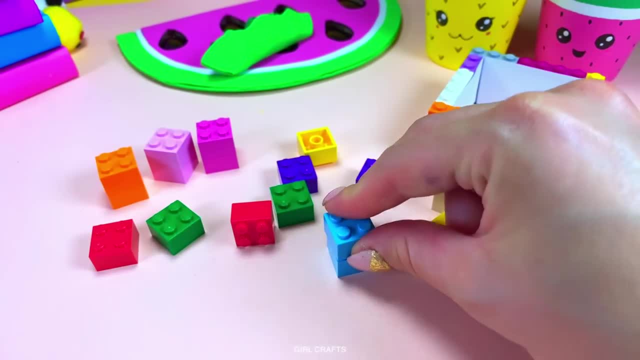 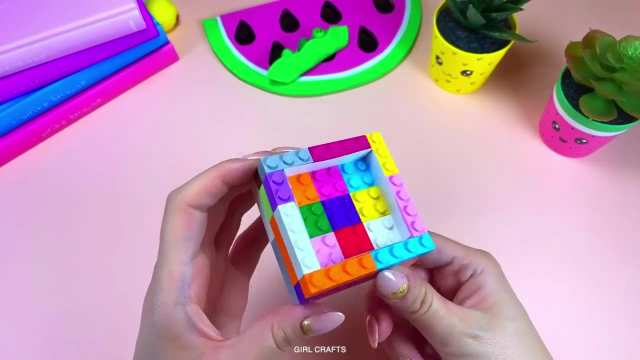 It's my show. you can get in for free. I'm who they're trying to beat. Wanna get on my team? Yeah, that's me. that's me. Got my swag on max. I'm a savage relax. Got my swag on max.